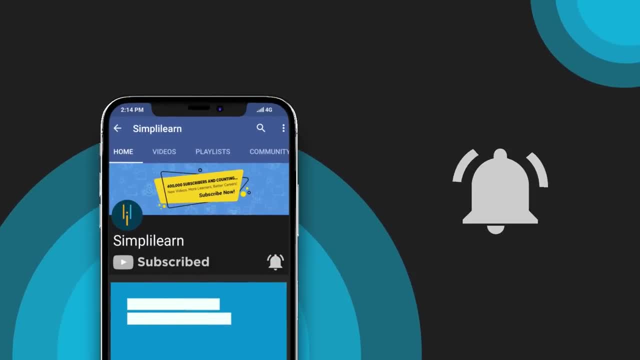 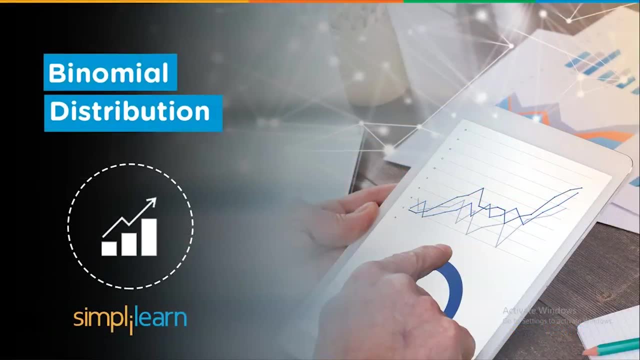 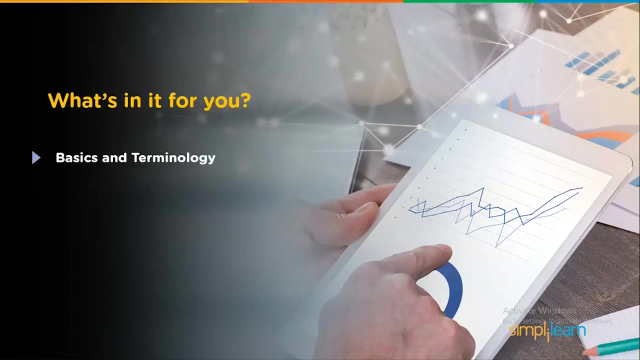 Hey everyone, Welcome to Simply Learn's YouTube channel. In this session, we'll discuss binomial distribution, which is an important topic of probability distribution. Let's discuss what's in it for you. We'll start this tutorial by discussing the important terms that you should know. Then we'll move on to discuss binomial distribution and 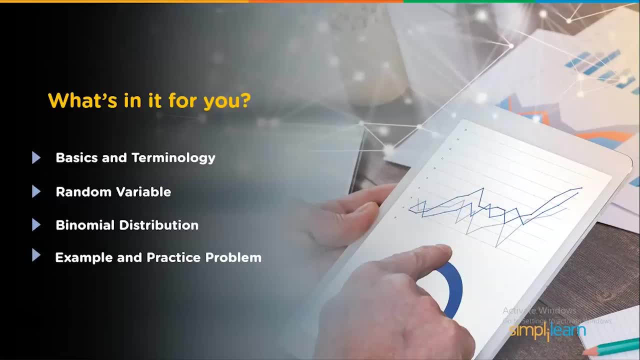 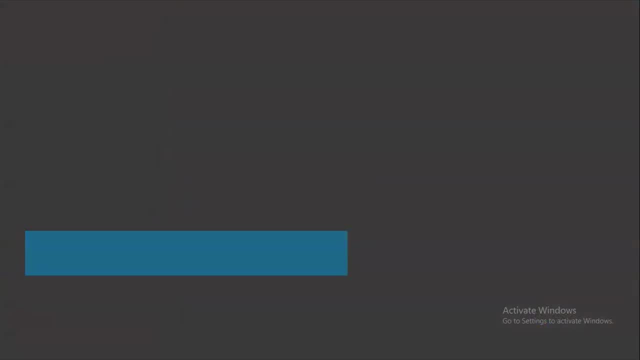 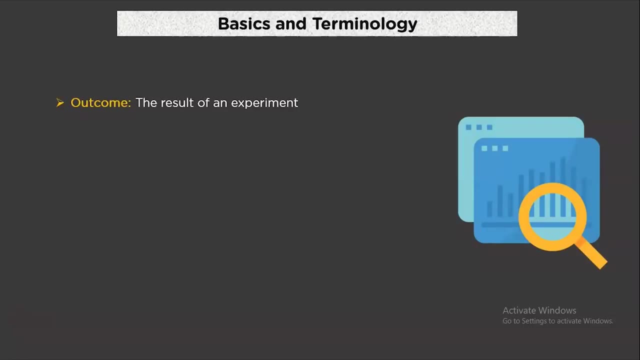 the formula for calculating the binomial coefficient. Then we'll work on an example to get the clear understanding of the topic. So let's get started. Basics and Terminology. The first one is Outcome. Whenever we do an experiment, like flipping a coin or rolling a dice, we get an outcome. For example, if 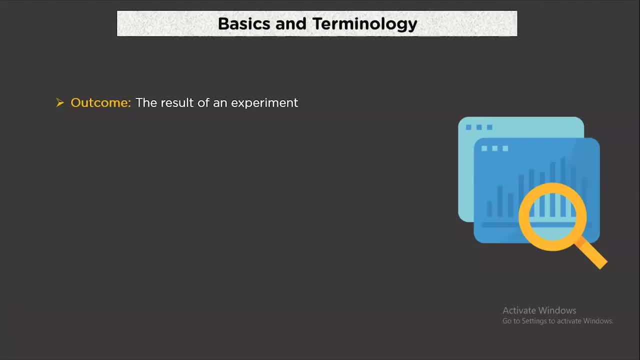 we flip a coin, we get an outcome of heads or tails, and if we roll a die, we get an outcome of 1,, 2,, 3,, 4,, 5 or 6.. A random experiment is any well-defined procedure that produces an observable outcome. that could 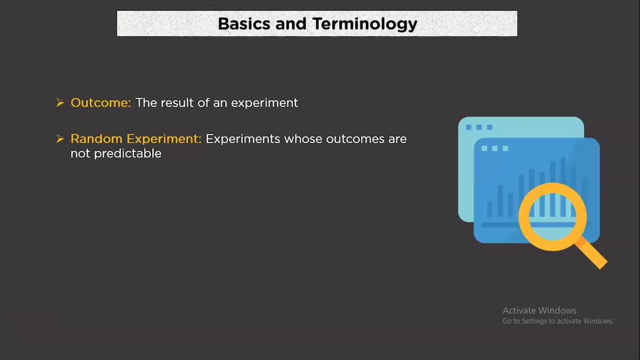 not be perfectly predicted in advance. A random experiment must be well-defined to eliminate any vagueness or surprise. It must produce a definite, observable outcome so that you know what happened after the random experiment is run. Random Events: Consider a simple example. Let us say that we 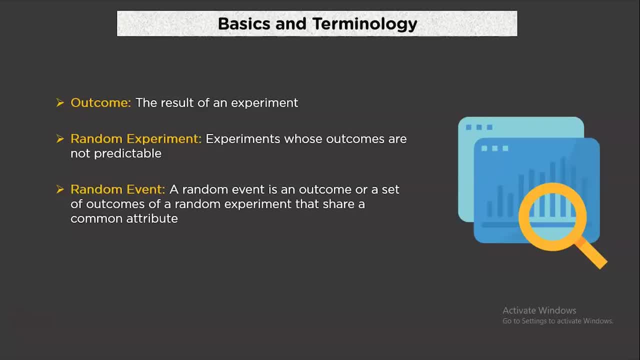 toss a coin up in the air. What can happen when it gets back? It either gives a head or a tail. These two are known as outcome, and the occurrence of an outcome is an event. Thus, the event is the outcome of some phenomenon. 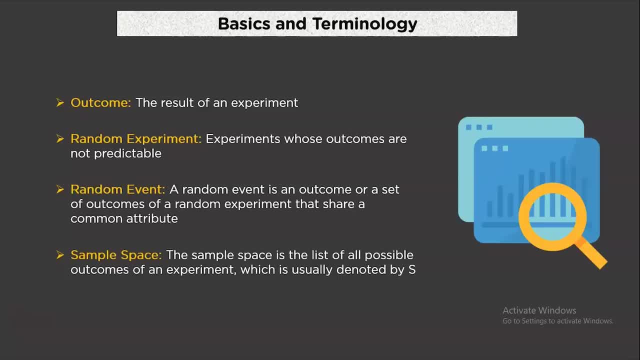 The last one is Sample Space. A sample space is a collection or a set of possible outcomes of a random experiment. The sample space is represented using the symbol s. The subset of all possible outcomes of an experiment is called a sample space, The sample space. 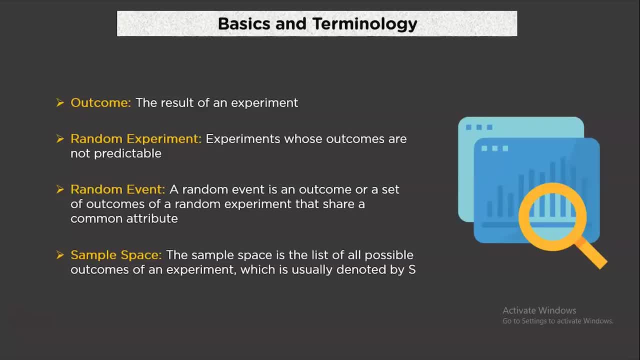 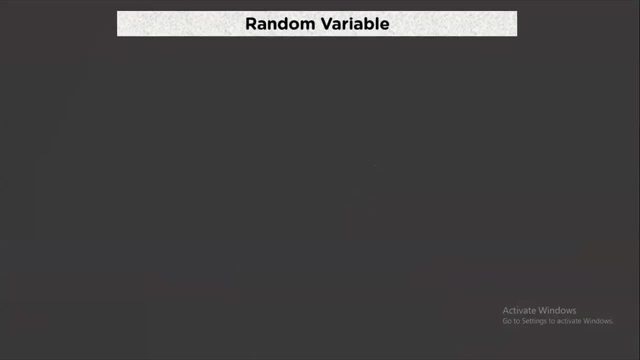 is a collection or a set of possible outcomes of a random experiment. The sample space is represented using the symbol s and contains an outcome that is a level to the amorphous makeshift expression or difference. Therefore, thisести is the output of the research experiment. 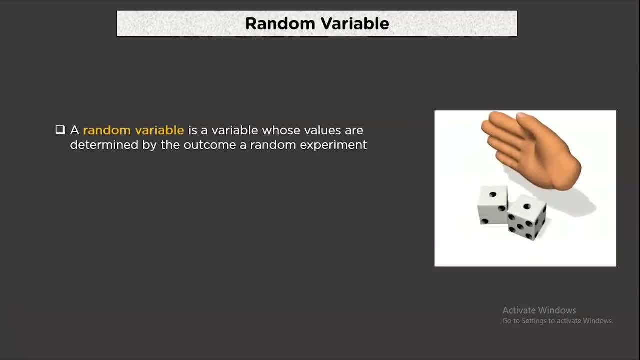 A random variable is a numerical description of the outcome of a statistical experiment. A random variable that may assume only a finite number of values is said to be discrete, Ie a randomestial system assume any value in some interval on the real number line is said to be continuous. 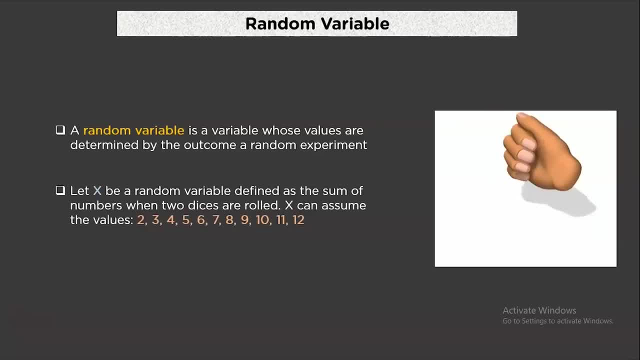 Let's see an example. Let x be a random variable defined as the sum of numbers. when two dices are rolled, x can assume the values 2, 3,, 4,, 5,, 6,, 7,, 8,, 9,, 10,, 11 and 12.. Notice there. 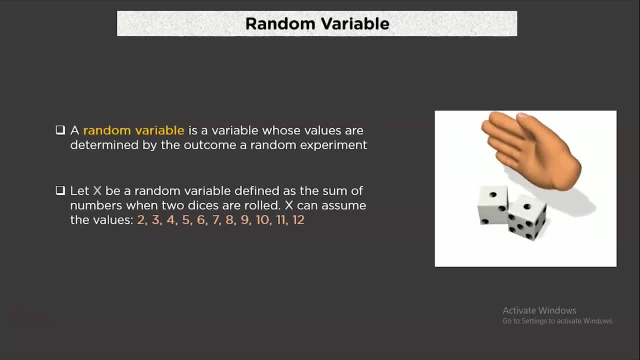 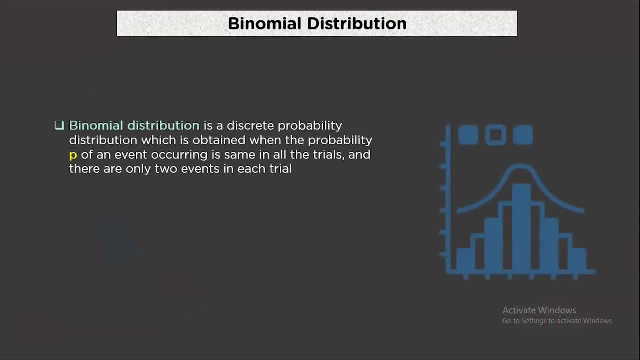 is no 1 here, because the sum on the two dice can never be 1.. Now that we know the basics, let's move on to binomial distribution. The binomial distribution is used when there are exactly 2 mutually exclusive outcomes of a trial. These outcomes are appropriately labeled: Success and Failure. The binomial 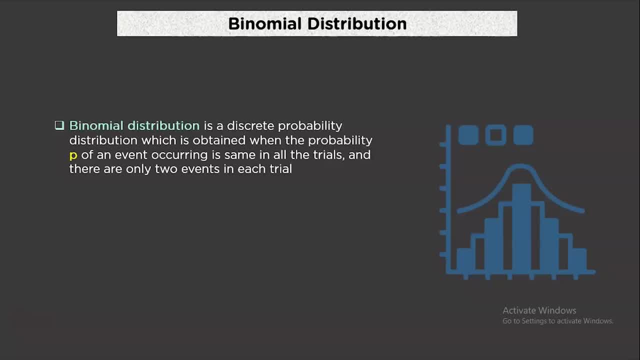 distribution is used to obtain the probability of observing x successes in n numbers of trials, with the probability of success on a single trial denoted by p. The binomial distribution assumes that p is fixed for all the trials. Here is a real-life example of a binomial distribution. Suppose you purchase a lottery ticket, then either 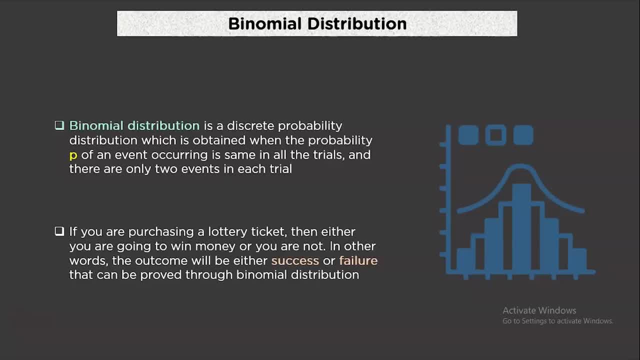 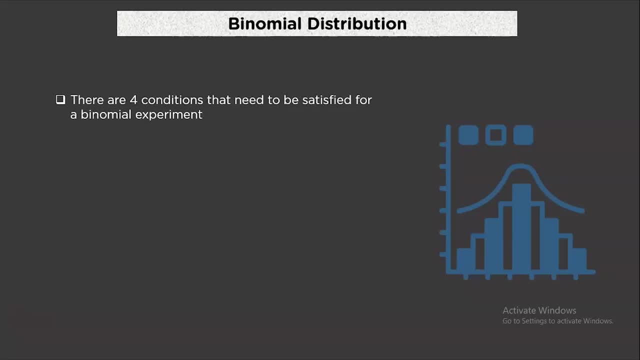 you are going to win the lottery or not. In other words, the outcome will be either success or failure. that can be proved through binomial distribution. There are four important conditions that needs to be fulfilled for an experiment to be a binomial experiment: 1. There should be a fixed number of n trials. 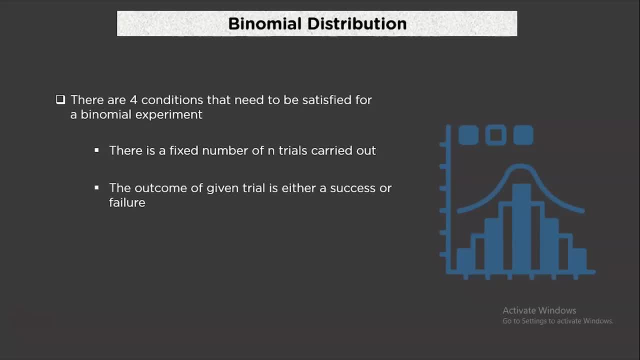 carried out. The outcome of a given trial is only 2. that is either a success or a failure. The probability of success remains constant from trial to trial. It does not change from one trial to another And the trials are independent. The outcome of a trial is not affected by 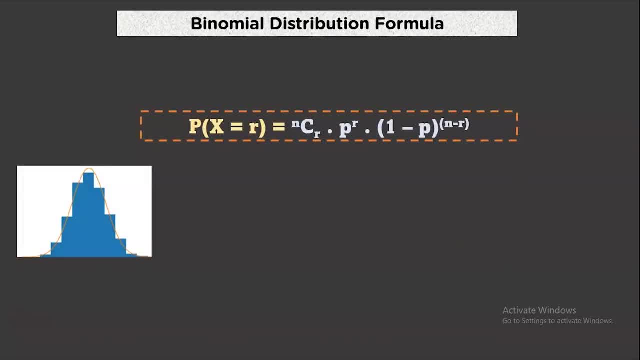 the outcome of any other trial. To calculate the binomial coefficient we use the formula, which is: nCr into P to the power r into, Where r is the number of success in n number of trials and p is the probability of success. One minus p denotes the probability of a failure. 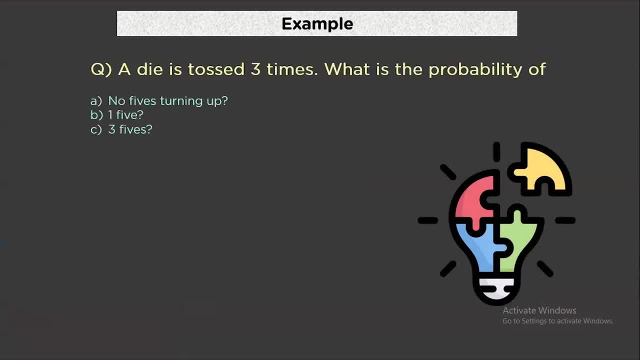 Now let's use this formula to solve an example. Suppose a die is tossed three times. What is the probability of no-5 turning up, one-five and three-fives turning up? To calculate the no-5 turning up here, r is equal to zero and n is equal to three.